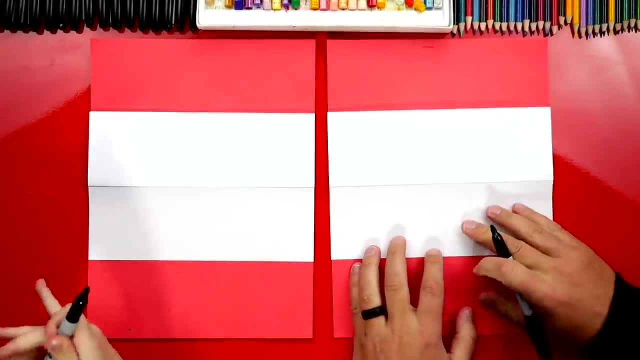 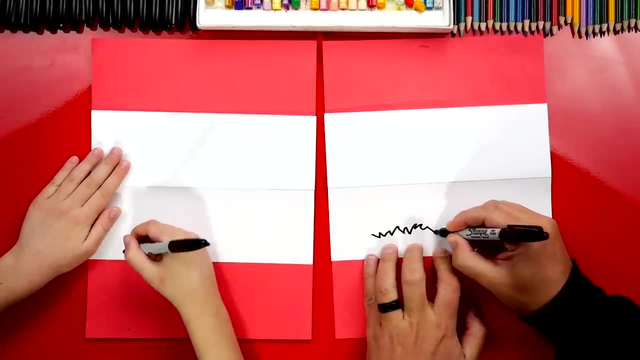 We're going to first draw the grass down here on the bottom of our paper, and I'm going to draw a zigzag line, and then I'm going to fold it down. I'm just going to draw a zigzag line, and yours doesn't have to look like mine. 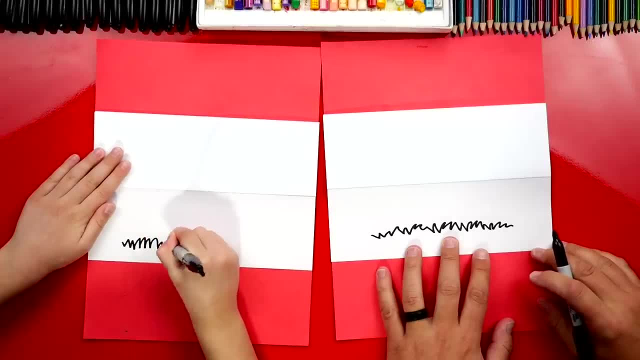 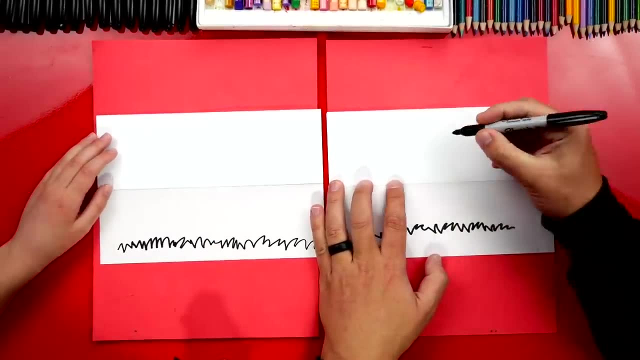 I'm just going to draw crazy grass There you go All the way across. Next we're going to draw the Easter egg. We're first going to draw the top part of our Easter egg. We're going to draw an upside down U shape. 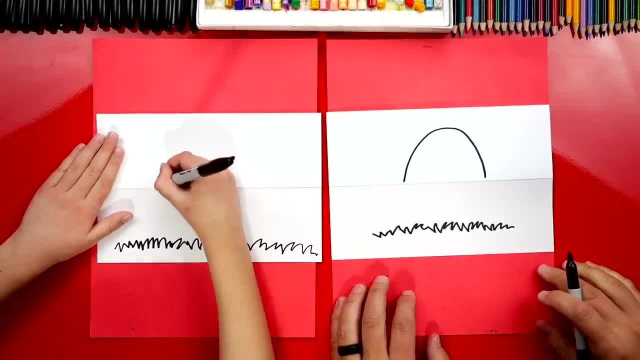 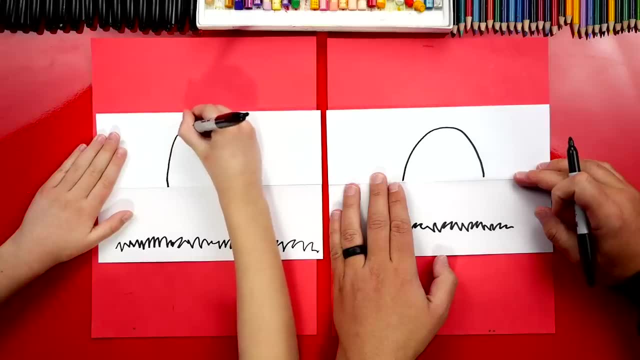 We're going to go up and then back down, and this is above the fold. Oh, I like the shape of your egg. It's going to be awesome. Oh, it's going to be a tall one, I like it. 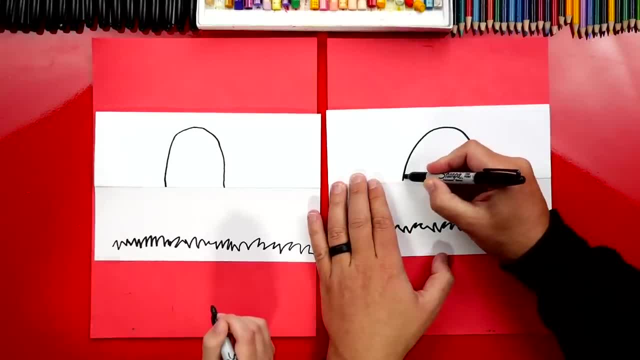 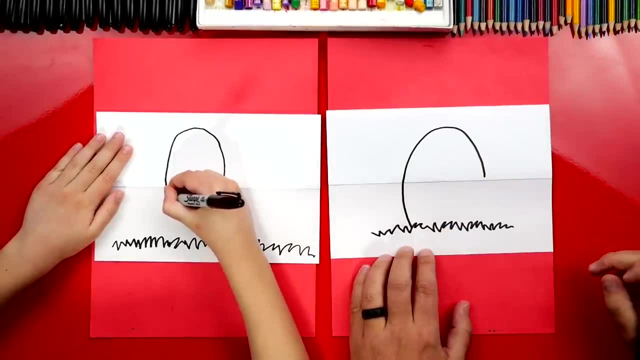 And skinny. Yeah. Now we're going to take each side of the Easter egg and we're going to extend it down and curve into the grass. So yours probably. yeah, there you go, I like it. Then we're going to draw the same thing on the other side. 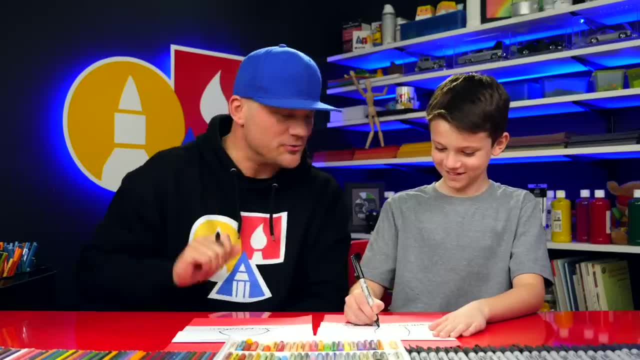 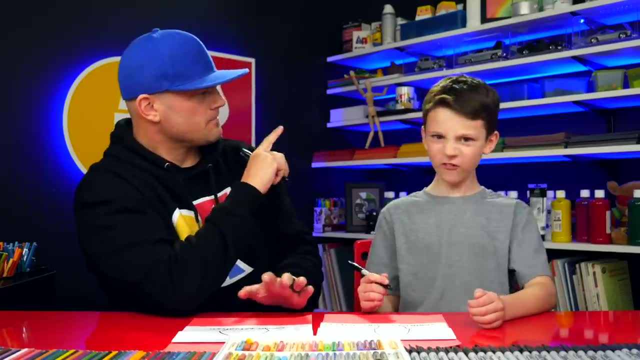 Extend it down and then curve it in. It's okay that our two drawings look different. I think your Easter egg looks perfect. The next time we draw it we could draw a little wider. The most important thing is To have fun. 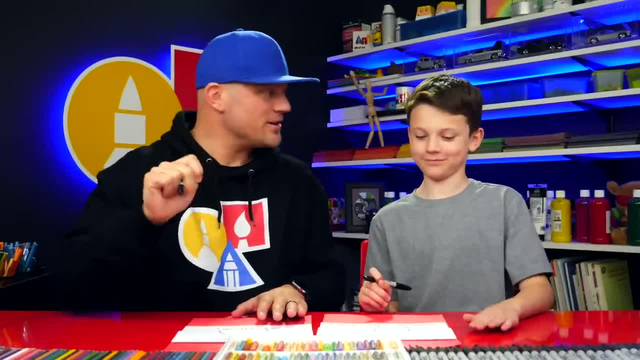 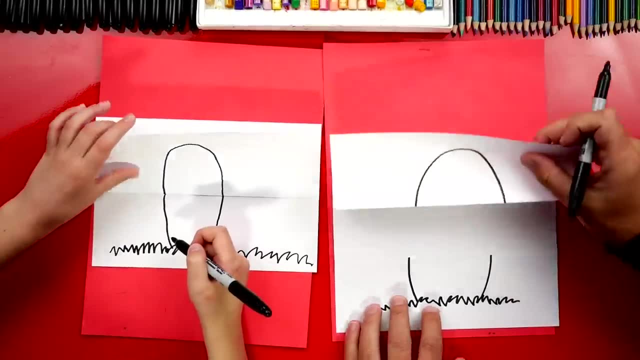 Yeah, to have fun and to Practice, Practice. I'm sure their drawings look different too, and that's okay. All right, let's keep going. Now we're ready to open up our drawing. We're going to unfold it and we'll flatten out the fold so it's easier to draw on. 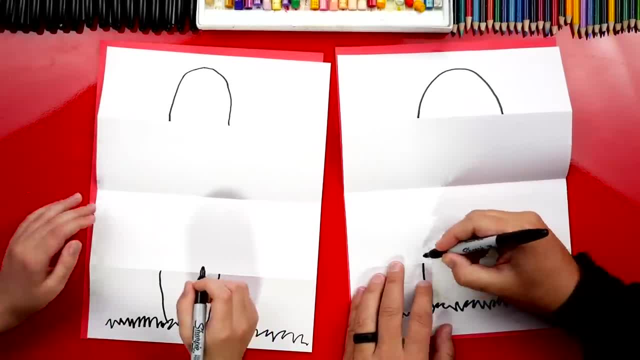 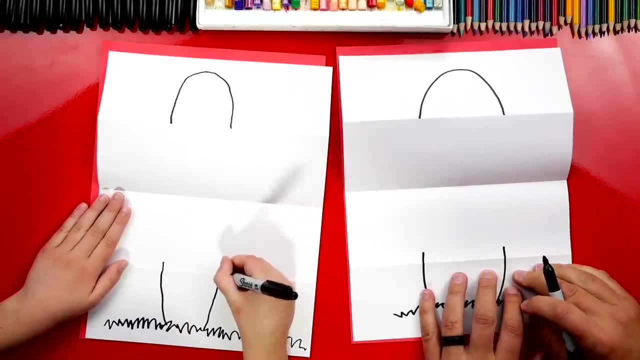 Now let's first start by finishing our egg. We're going to draw it cracked open. We're going to draw, extend the side up just a little higher, on both sides, down here at the bottom. Now this next part: we want to make sure that we don't draw below this bottom fold. 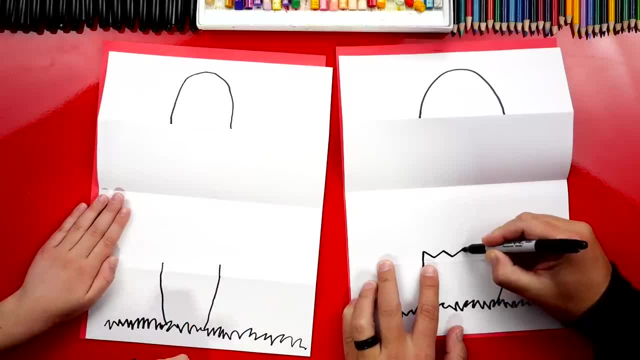 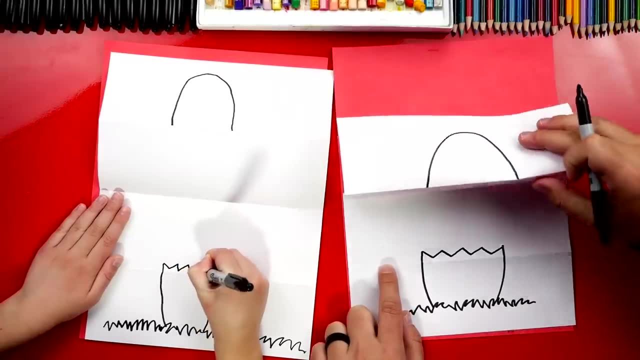 We're going to draw a zigzag line. Watch me, We're going to draw it all the way over to the other side. but we want to make sure that those little points don't go below the fold. That's because when we fold it back up, we want it to be hidden. 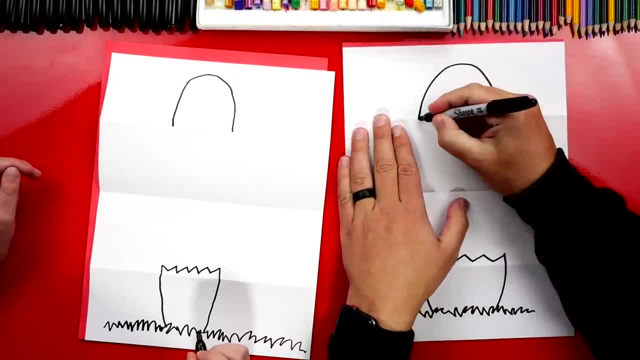 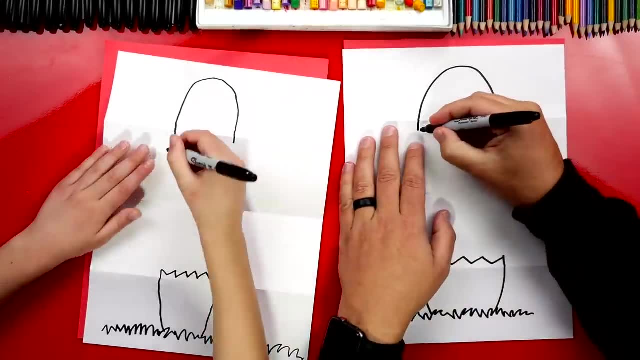 Okay, now we're going to repeat that same step, except up here at the top. So let's first extend each side further down, Yeah, and then we're going to draw a zigzag line and make sure that these little points don't go above the fold. 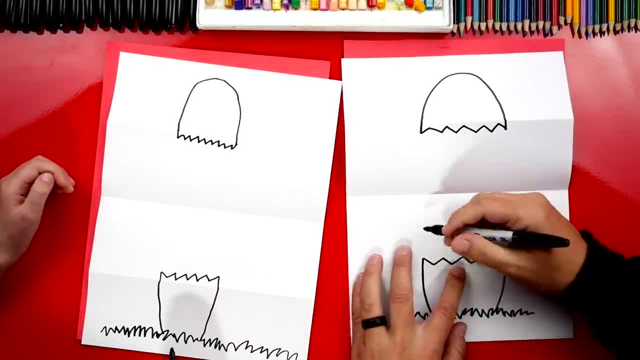 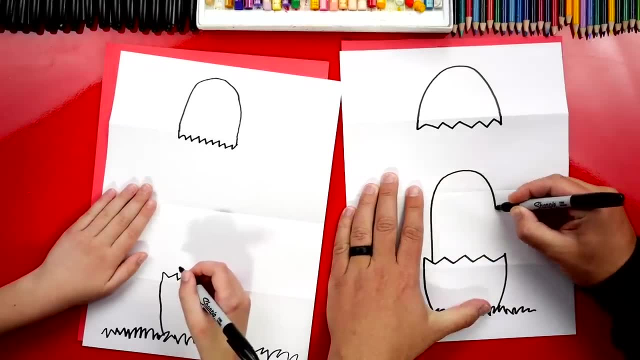 Yeah, all right, We did it. Now we're ready to draw our Easter Bunny. We're going to draw a really funny one. We're going to draw him coming up out of the bottom egg. I'm going to draw a big upside down U like that. 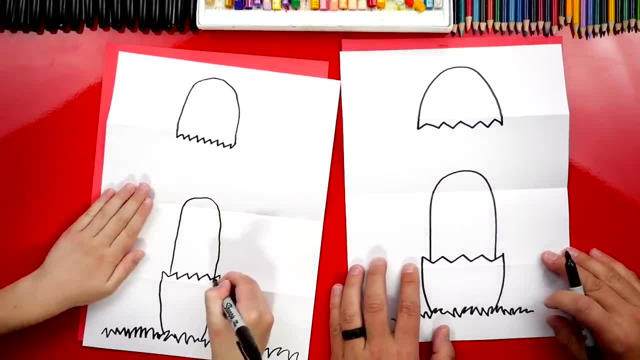 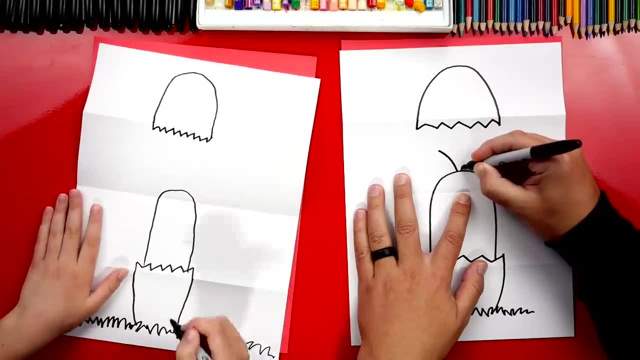 There we go. Good job, It's so skinny, I like it. Then we're going to draw Little bunny ears, So I'm going to draw a curve that comes out to the side or up and out. Both sides looks like a bug. 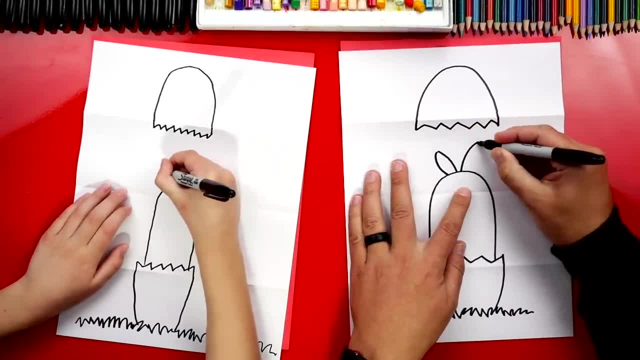 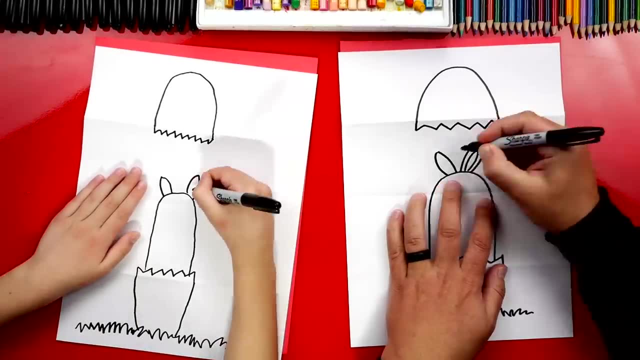 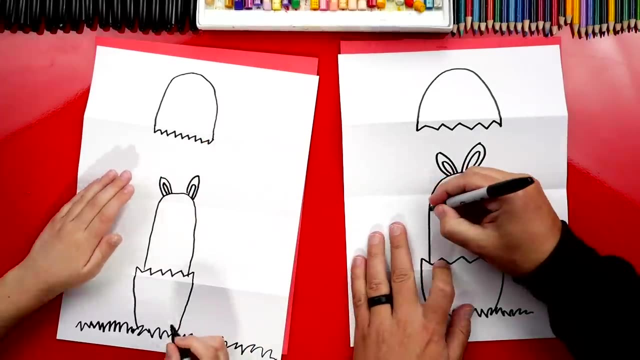 And then we're going to draw the other side of the bunny ear. coming back down on both sides, Let's draw the inside of our bunny ears. We'll draw that same shape, but smaller on each ear. Okay, let's also draw little arms sticking out. 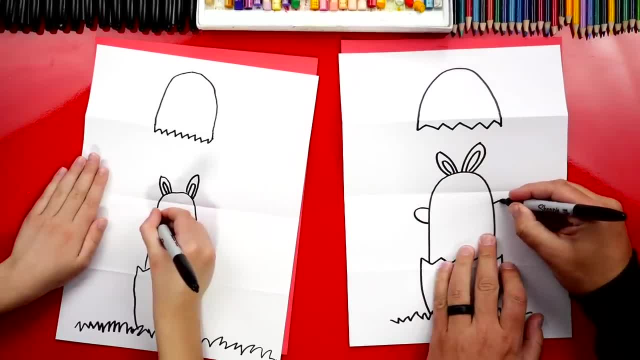 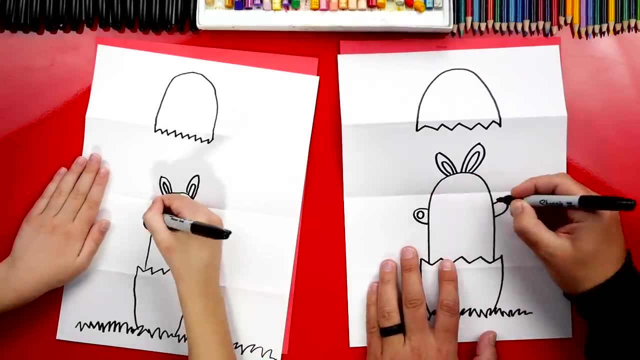 So I'm going to draw Sideways U shape over here and a sideways U shape on the right. Oh, we can also give him. Let's give him a little paw circle on the left and a circle over here on the right. Next, let's draw his eyes. 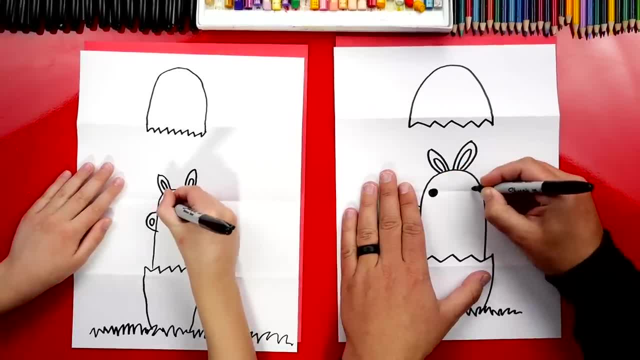 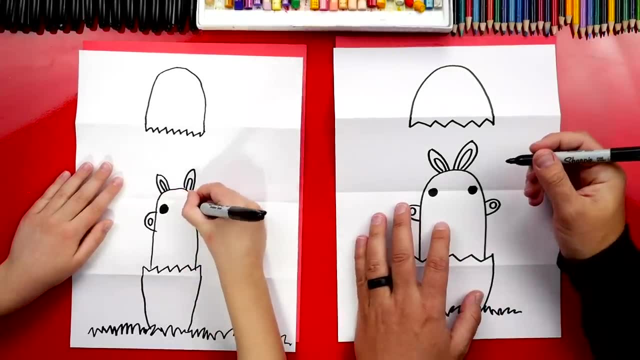 I'm going to draw a small little circle, Color it in and a smaller little circle over here and color that one in also, And then we can. Oh yeah, Keep going, Then we could draw his mouth. I'm going to draw a little. 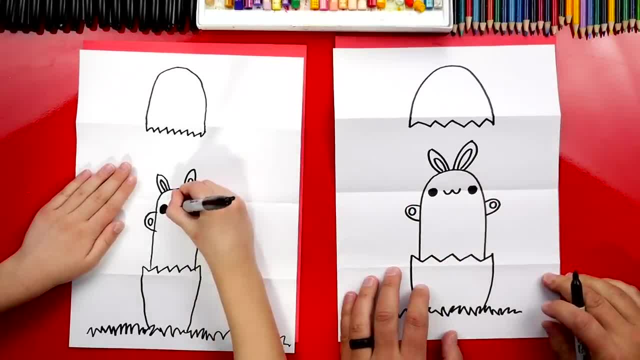 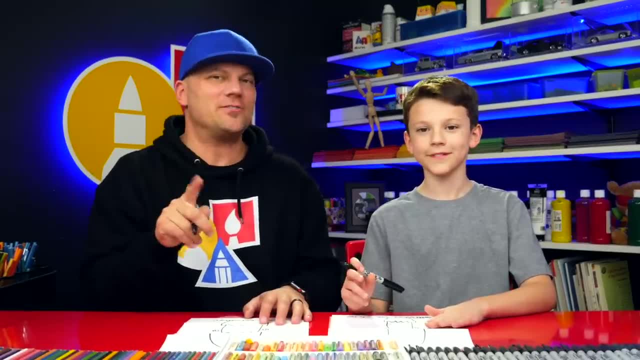 Curve, Curve, Curve W in between the eyes. If we ever go too fast, what can our friends do? Pause the video? Yeah, If we fast forward the video or if we go too fast and you need extra time, Remember you can always pause the video. 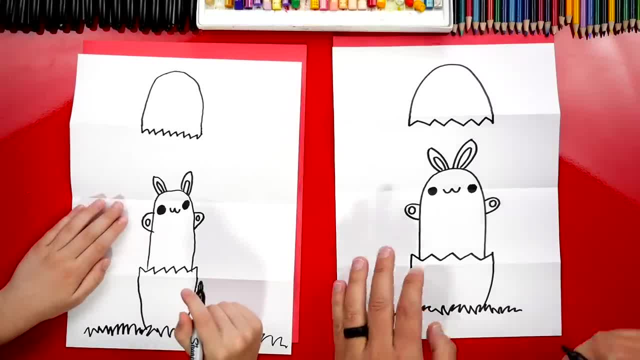 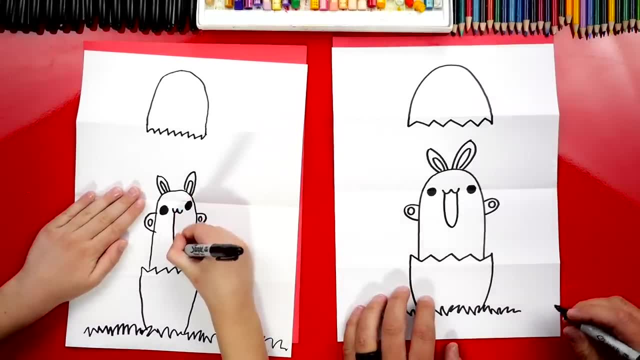 All right, What else should we draw? Let's make his mouth bigger. Oh, okay, Let's do that. I'm going to draw a big U shape for his mouth, and we could also give him bunny teeth. right, I'm going to give him bunny teeth. 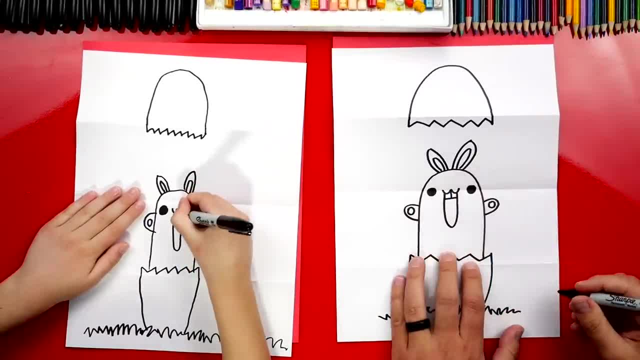 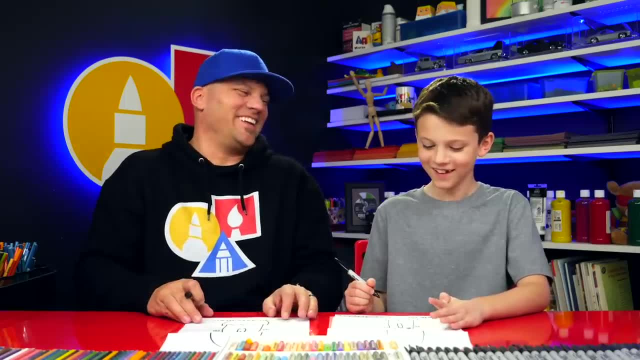 I'm going to draw a line up At the top and then a line right down the middle, and we could also give him a tongue. It's a beaver. Yeah, Well, it's a bunny, but that's okay. Now we did it.